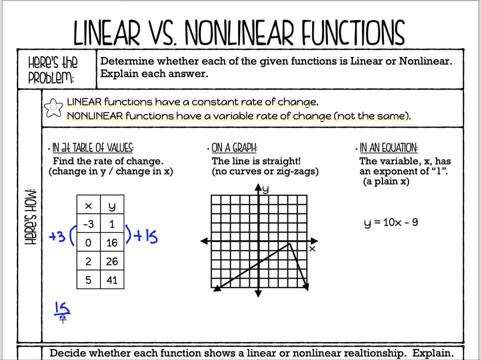 over. my change in x is going to be 15 over 3, and that equals 5.. All right, let's try the next one. I'll be colorful: From 16 to 26,- that's a plus 10, and over on this side, from 0 to 2, that's a plus. 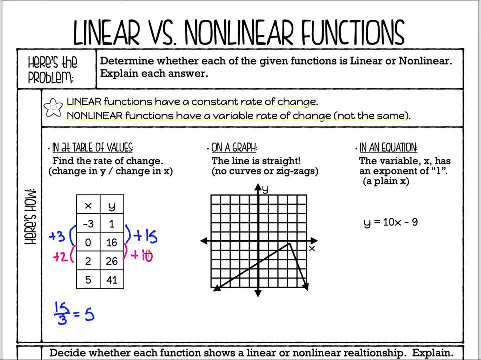 2.. So you might look at this and think, oh, this isn't linear because this is different. However, be careful, You've got to check your change in y over your change in x and if we do 10 over 2,. 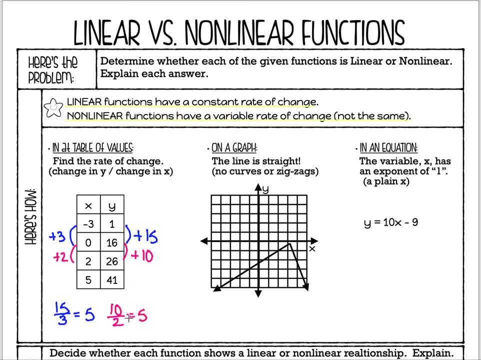 that is 5.. Right, So it's the same thing, same rate of change. All right, then we can check our next one From 26 to 41, so that's a plus 15 again. Well, since this is a plus 15, this better be a. 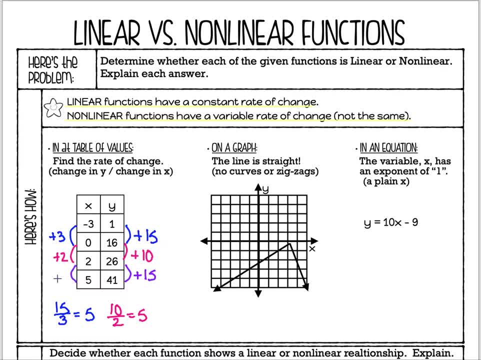 plus 3 over here, or it's not going to work. Fortunately, 2 plus 3 does give us 5.. So we've got 15 over 3, and again that is positive 5.. So these all have the same rate of change. 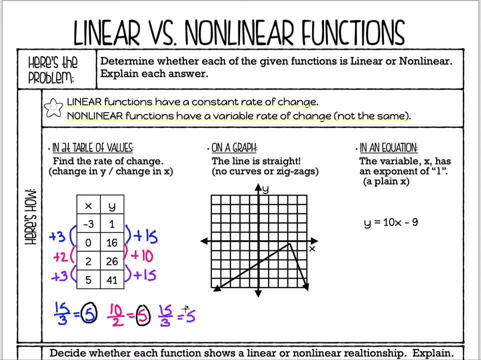 right. We've got a rate of change of 5 every single time And you have to make sure you check the whole table because the first two might work and then maybe the third one doesn't, and then that means it's not a constant rate of change. So this is going to be a linear function. 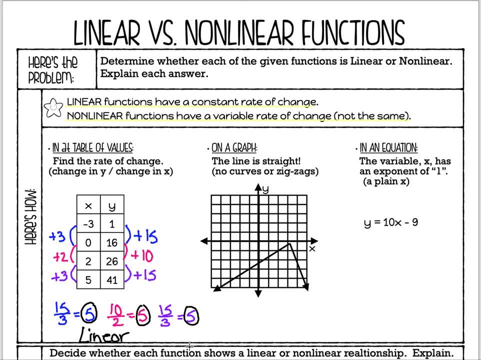 right here and that's because it's got the same constant rate of change. All right, then we're going to look on a graph Now. on a graph, the way that we're going to know that a function is linear is it's going to be a straight line, right. 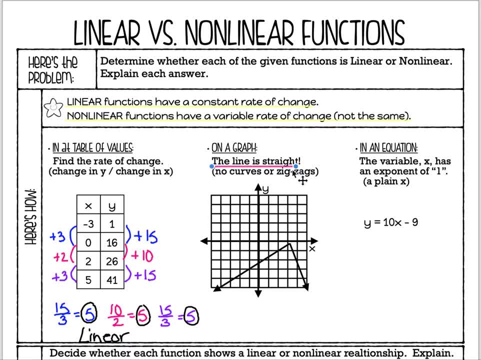 Line is straight, And you have to be careful with this. It means one continuous straight line. It doesn't mean a straight line going up and then a straight line going down. right, No zigzags. okay, No curves. no zigzags. So this one is going to be nonlinear. Whoops. And the reason that this. 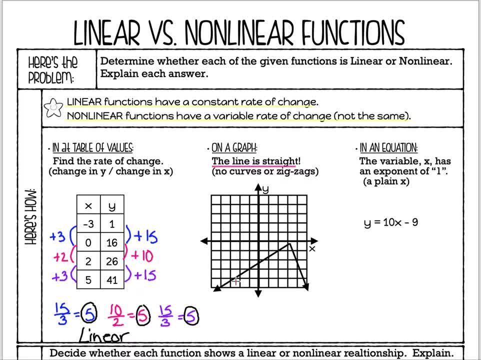 is nonlinear is because the line is going up and then it's coming down, right, So this is nonlinear. So be careful: Even though it's made up of two straight line segments, that does not mean it's linear. It's got to be one continuous line. 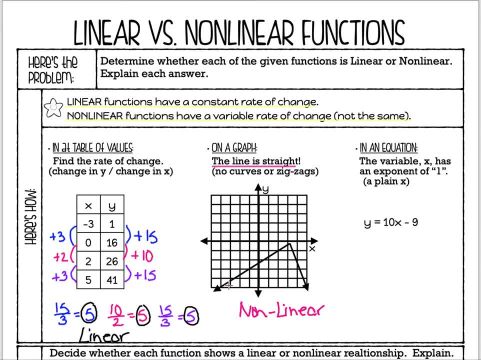 And another way we can think of it, as this line is going up here, right, So this would have a positive slope, and then it's coming down, So this is going to be a negative slope. So if something has a positive slope and then a negative slope, that's not the same rate of change. 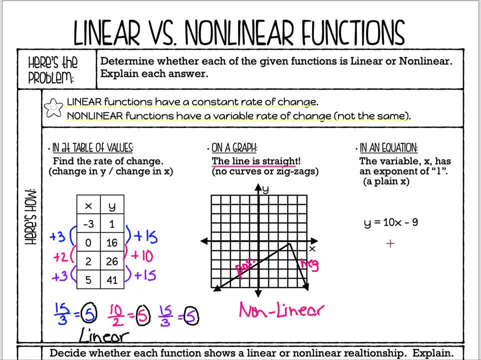 All right, then we've got an equation. So when you have an equation, all you're doing is you are looking at whatever exponent is on the x, right? So we're going to look at the variable x, We're looking at this x right here, And we're going to look at what exponent is on the x And we want it to have. 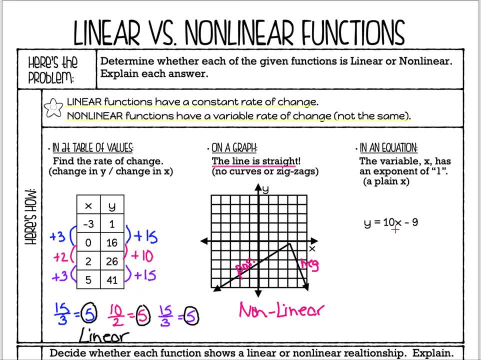 an exponent of 1.. Now we know that whenever we have a plain variable- when I have a plain old x here- that really means x to the first power, right? We just don't bother to write it. So because this is a plain x or an x to the first power, that means this is linear. 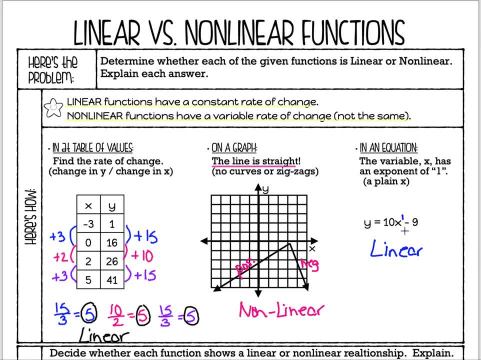 And that's it right. If we were to graph this line, we would put a point on negative 9, right, Because that would be our y-intercept, And then we'd be going up 10 and right 1, up 10, right 1, up 10, right 1.. So that would be a constant rate of change. 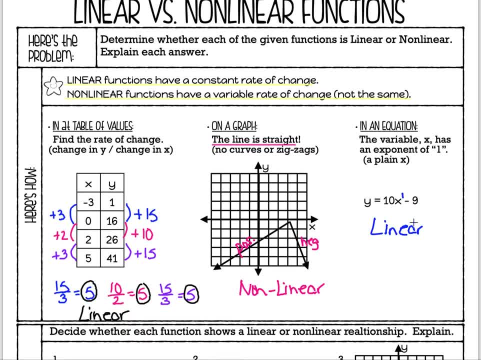 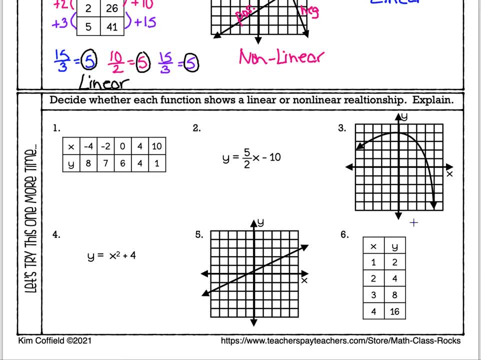 All right, let's look at these examples on the bottom. Now, if you're feeling good about this and you want to try to do these six problems on the bottom, why don't you do that? You can stop the video while you do it and then start playing it again, And then we'll go over. 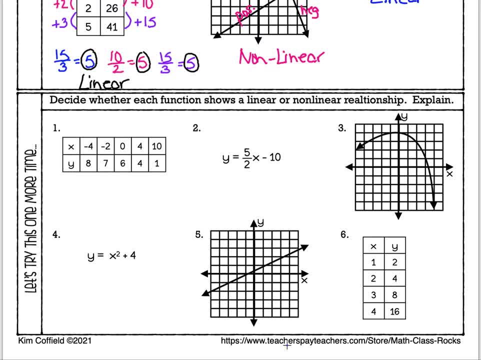 the answers together. So if you're feeling good about this and you want to try to do these six together, If you're feeling confused and you want to watch me do a few more, I am fine with that as well. All right, here we go, Number one. So we're going to figure out our change in y over. 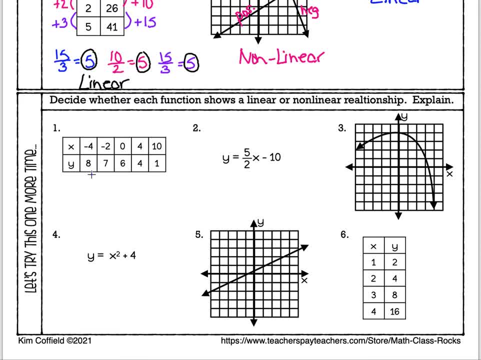 our change in x and we need to check the whole entire table. So from 8 to 7, we've got a minus 1.. From negative 4 to negative 2, we've got a plus 2. From 7 to 6, we've got a negative 1.. 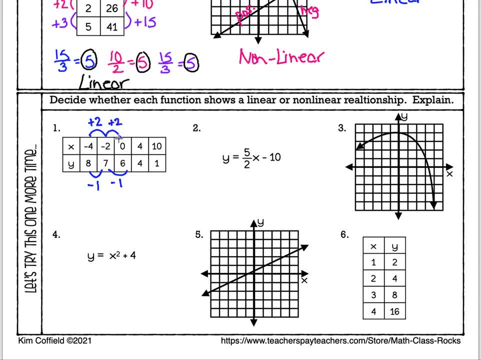 From negative 2 to 0, we've got a plus 2.. From 6 to 4, we've got a negative 2 this time, And from 0 to 4, we have a plus 4.. And then, from 4 down to 1, we've got a negative 3 this time, And from 4 to 10, we have a plus 6.. 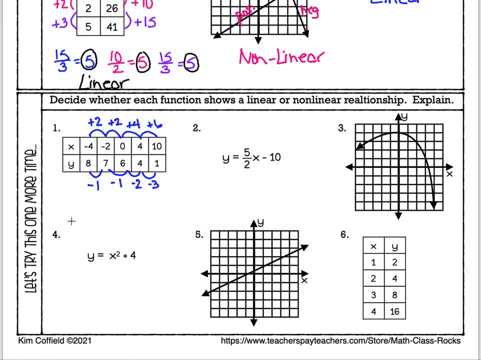 So we need to check all of these change in y over change in x. So I've got negative 1 over 2, right Negative 1, half Same thing again, negative 1 over 2.. Here I've got negative 2. 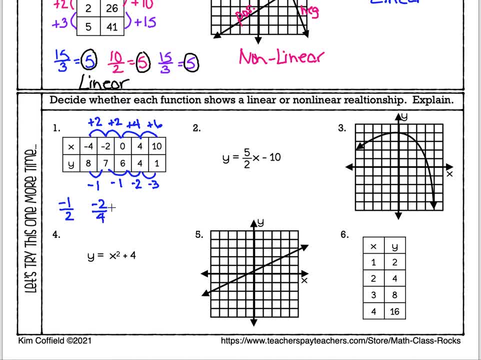 over positive 4.. Well, negative 2 over positive 4, if I reduce that would be negative 1 half, So that works. And then here we've got negative 3 over positive 6, which again will reduce to negative 1 half. So when I look at these rates of change, they're all the same, right, They are all. 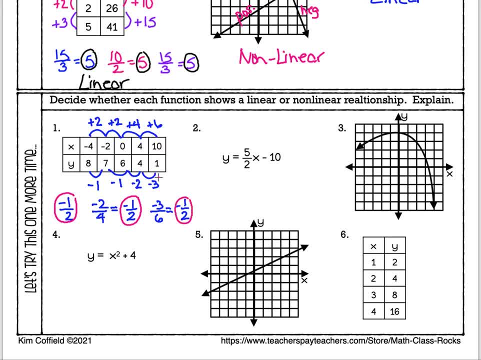 negative 1 half. Even though the numbers in the table were a bit different at times, they all reduce to the same thing. So that means that we're going to have a negative 1 half. So we're going to that. this is actually linear because it's got the same rate of change. So I'm going to write a. 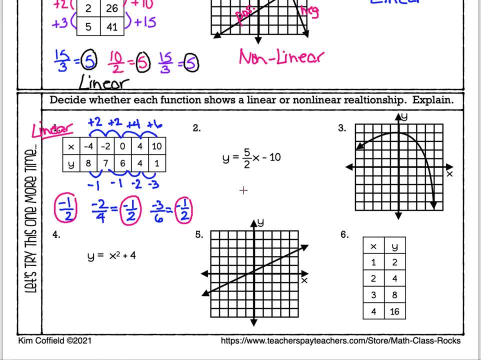 little note here that this one is linear. All right For an equation. remember, all you're doing is looking at the exponent that is on the x. Well, here's my x. I say to myself: is that a plain x? It certainly is right. If this had an exponent on it, it would just be an exponent of 1.. 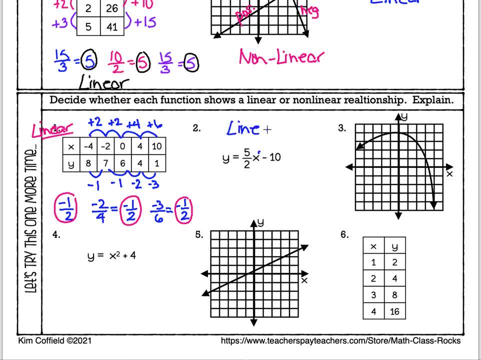 So this one is linear, All right. So for this one, hopefully we can tell that this graph is not linear right, Because it does not make a straight line, a continuous straight line. We've got a big old curve in here, So this one is. 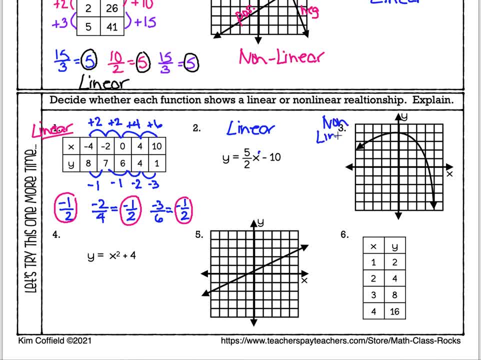 nonlinear, And my reason for that would be my line is curved right. This big curve right here tells me right away that it is not linear. All right, So for this equation down here again, I'm looking at my x and I'm checking that exponent. Well, 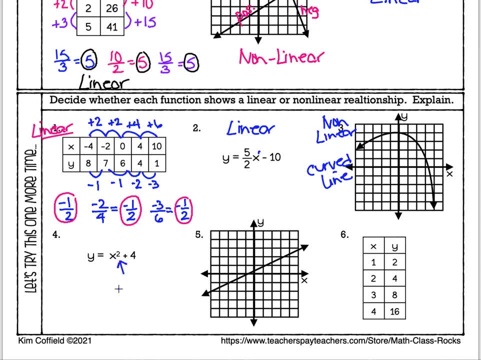 look at this. This one has an exponent of 2, right, The exponent is 2.. So, because that has an exponent of 2 and it doesn't have a plain old x or an x to the first power, that means this is: